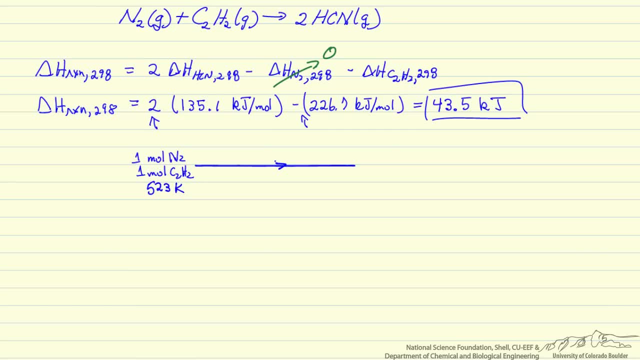 The idea is we are starting out with a mole of nitrogen, a mole of acetylene. We are at 523 Kelvin. We are going to form 2 moles of HCN at 523 Kelvin And we want to know what is the heat of reaction at 523 Kelvin. So what we are going to do is say: let's cool. 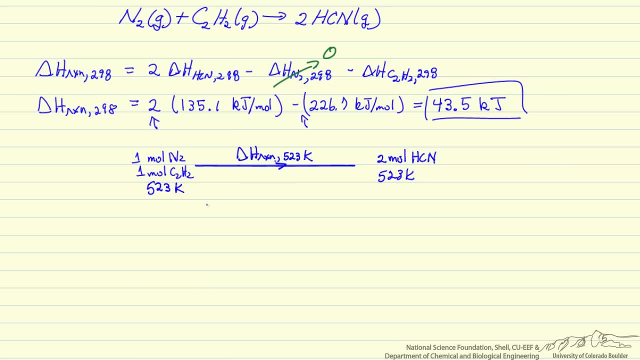 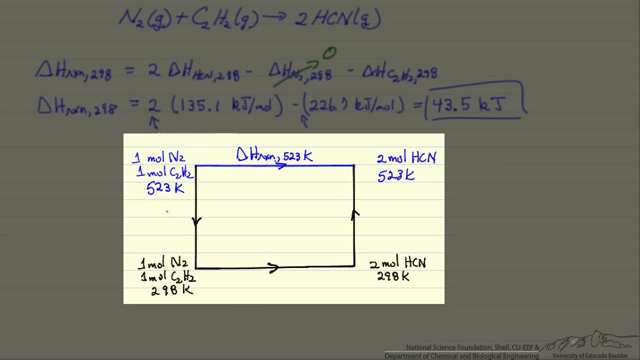 the reactants down to 298.. We can calculate that energy change from heat capacities Carry out the reaction at 298 and then heat them back up to 523.. So what I have drawn is an alternate pathway then in black, where first we cool down our reactants and there is going to be some enthalpy change. 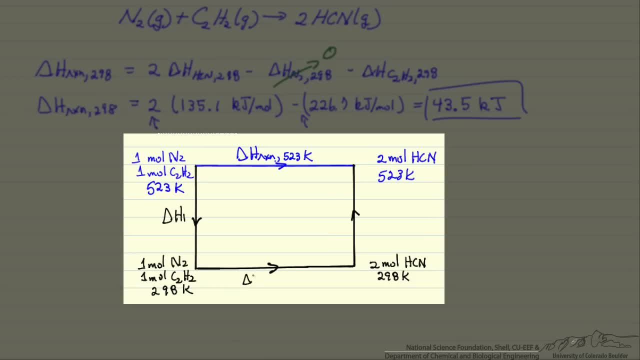 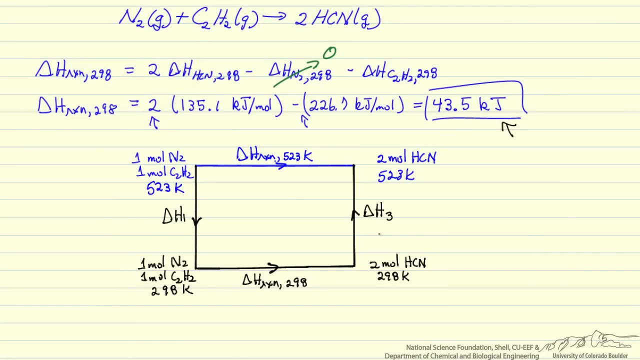 We are then going to carry out the reaction at 298.. So this is the heat of reaction at 298 which we are going to calculate it, And then we are going to heat the products back to 523. Called it delta H3. And the sum of the three delta H's, the black pathway, is going to be same. 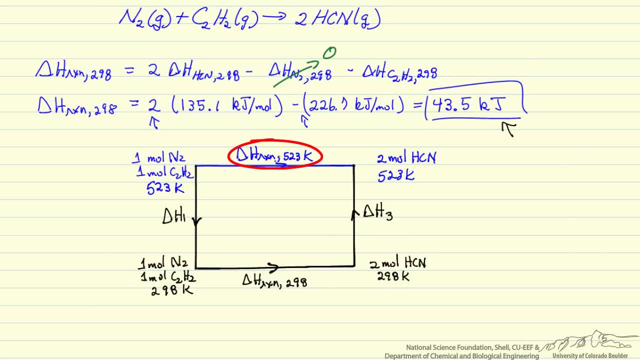 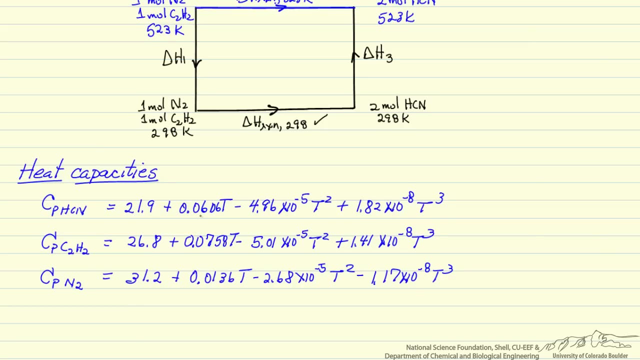 as delta H for the blue pathway for the reaction at 523.. And that is the value we want to determine. So we have this value. we need to calculate the changes from the heat capacities and the temperature change Over. here are the heat capacities as a function of temperature, where the temperature is in. 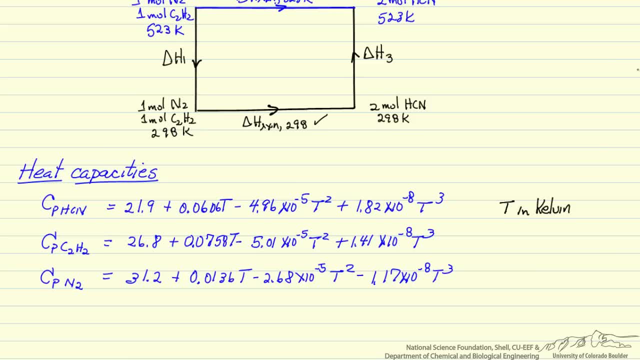 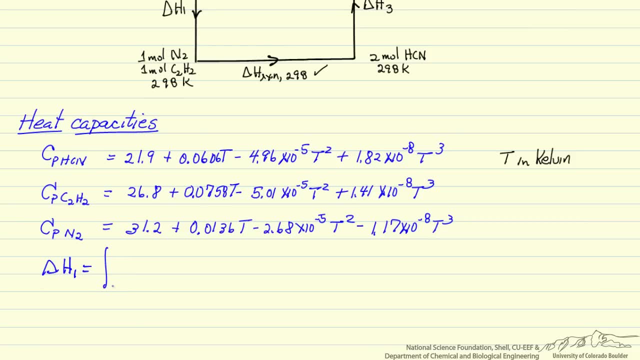 Kelvin. in these equations We will first calculate delta H1.. So delta H1 is going to be the integral from our starting temperature 523 to our final temperature 298.. The heat capacity of nitrogen plus the heat capacity of acetylene, And we are going to integrate over this. 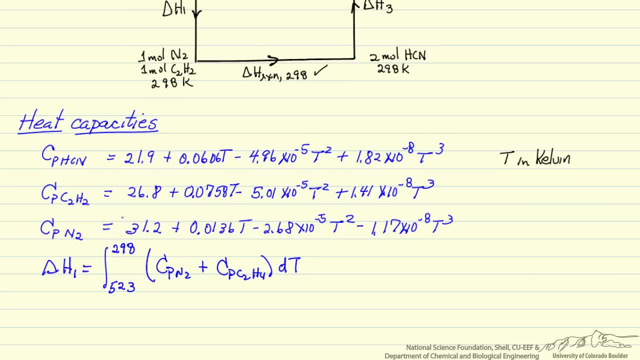 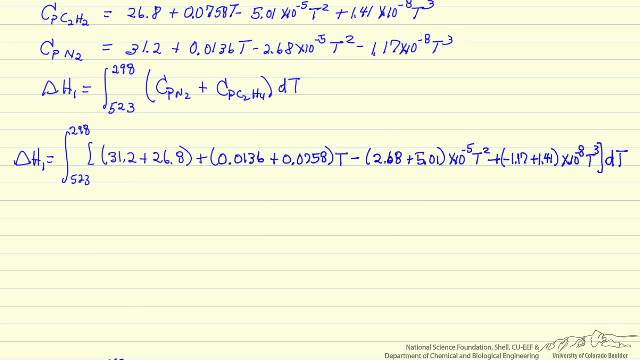 temperature range. So I am going to substitute in the values for the heat capacities and I am going to combine terms. I will combine this term plus this term for the first term and the integration and likewise for the other terms, And so we have four terms that we are. 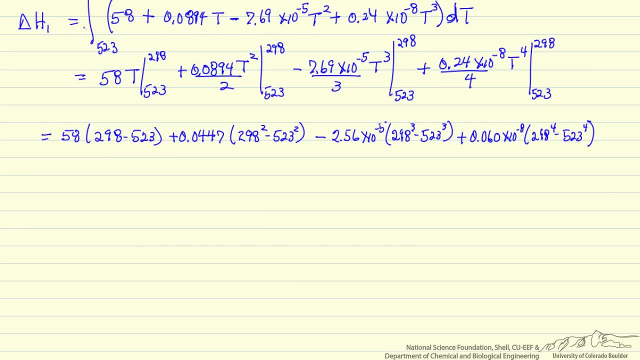 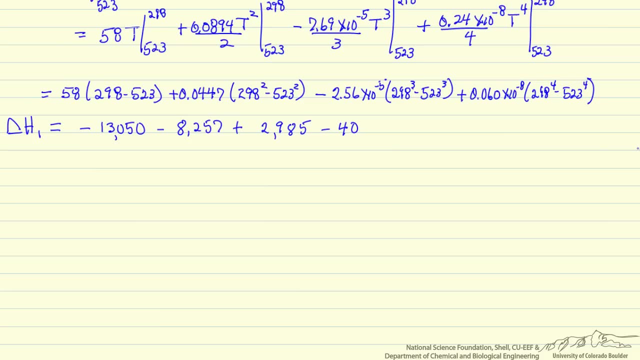 going to integrate. And then we have substituted in the limits for each of the terms, And now we will do the math to calculate each of these terms. This gives us a value for delta H1 of minus 18,362 joules, which is minus 18.4 kilojoules. 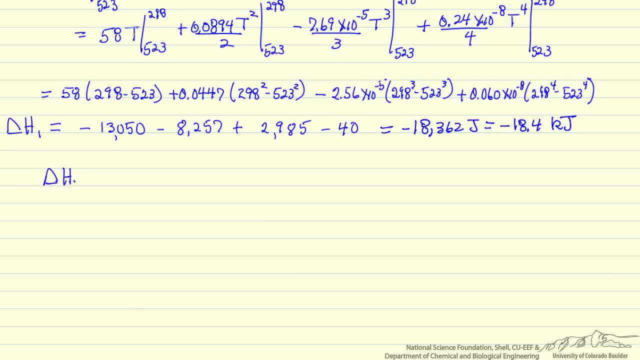 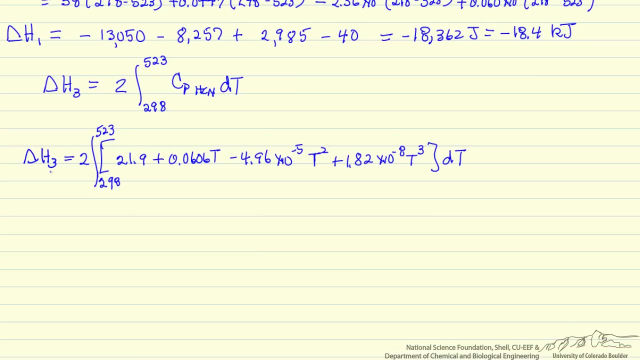 So now we are going to do the same calculation for delta H3.. Now we have two moles of HCN And we are now heating from 298 to 523.. And we only have one species. So we are going to substitute in the value for the heat capacity. So here is the heat capacity for HCN. We are 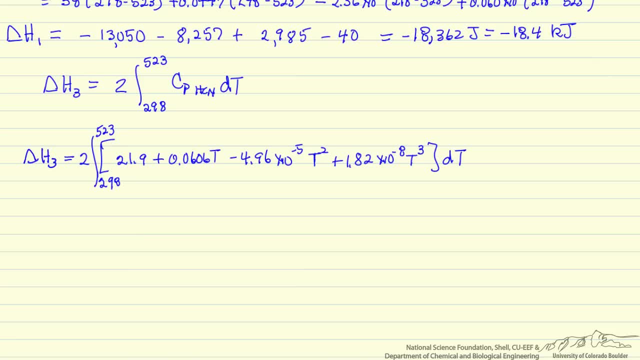 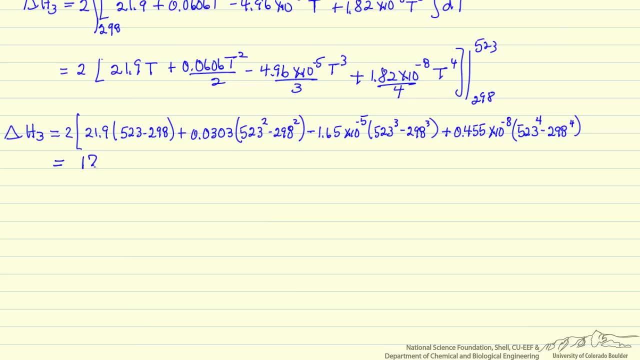 going to now do the same kind of integration as we did before And substitute in the limits The value of delta H3 is 17,580 joules or 17.6. if I round off kilojoules, So this is 1.610 joules And the H3 is the heat capacity, So delta H3 is 1.720 joules or 1.880 joules. 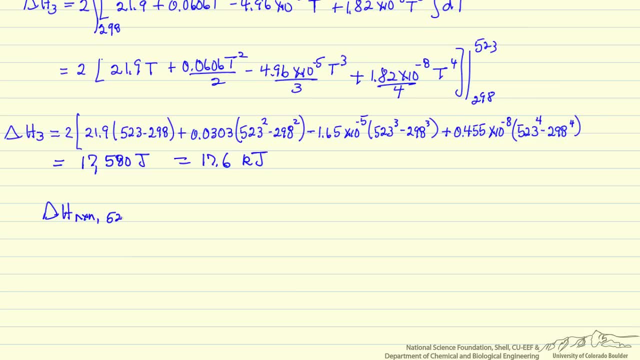 So delta H3 is 1.780 joules or 1.880 joules, And July 48th is the heat capacity. So delta H3 is 1.880 joules, but the H3 is 1.880 joules, So the value of H3 is 1.880.. So we are going. 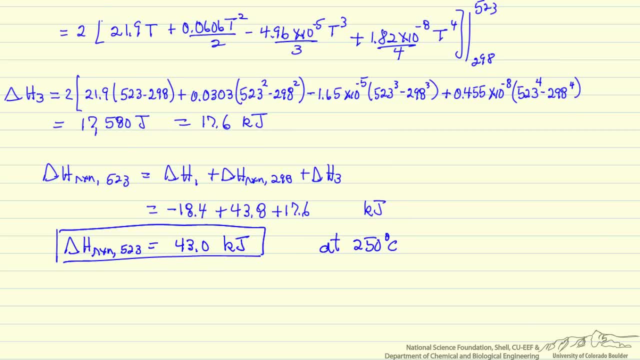 to subtract these three values in, So delta H reaction at 523 Kelvin is delta H1 plus delta H of reaction at 298 plus delta H3.. So I can substitute these three values in: And so delta H reaction at 523 is 43.0 kilojoules. This is per mole of acetylene reacting. Notice. 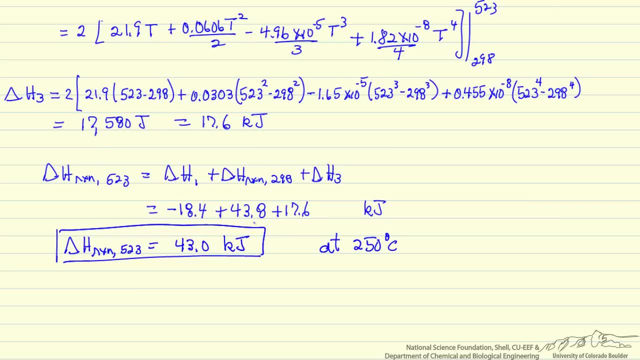 it is not very different from the 43.8 at 298.. So delta H reaction at 523 is one and 0 kilojoules, And this is fairly common, that these two heat capacity terms almost cancel out. so it's often that we assume the heat of reaction is not a function of temperature. 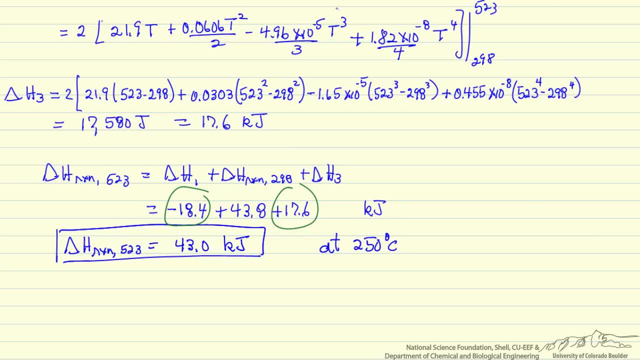 For this temperature range of 225 degrees C there's only a 1.8% difference in the heat reaction. Only delta H of reaction as constant is not a bad assumption in many cases.